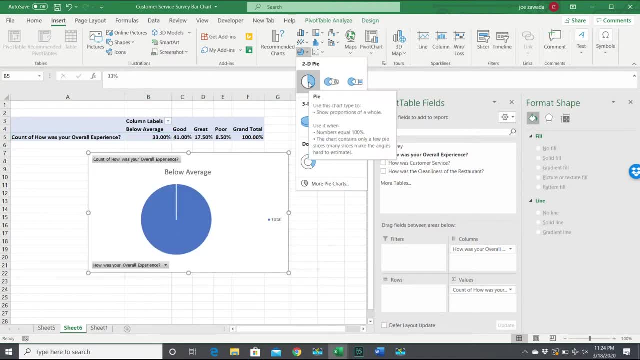 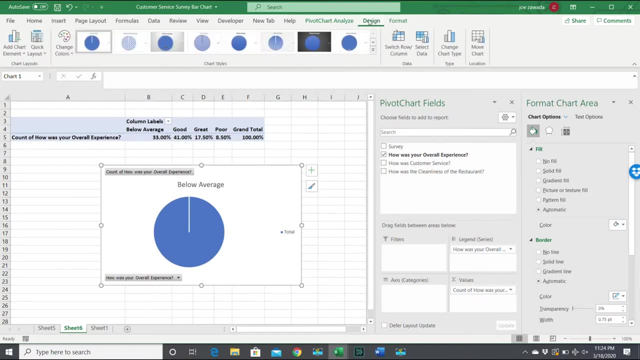 pie chart. we're just going to do a 2d chart to start. this doesn't really look like much, so we're going to need to switch things. so we're going to click on the design and we're going to need to switch the rows and the columns, and we do that. then we'll get our normal looking chart, because 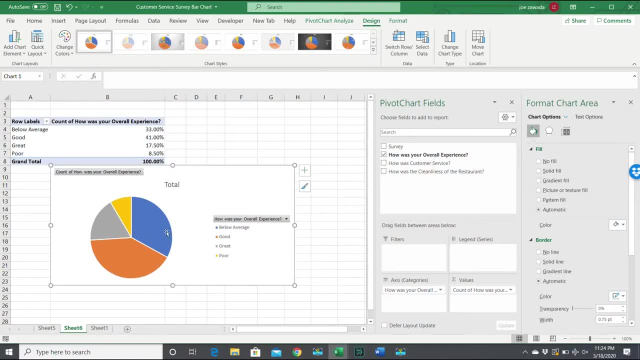 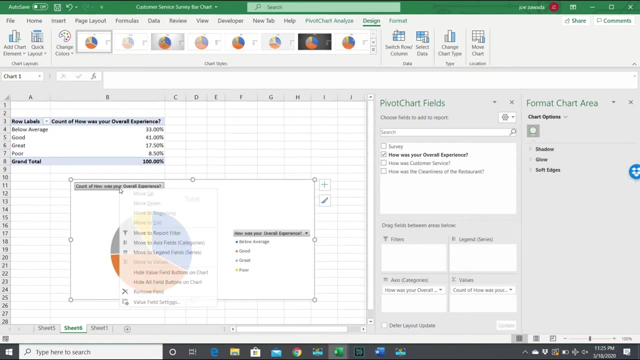 then the axis will change and then we have our, our data here. so we've got below average, good, great and poor. so let's format this table how we want to make it, to make it look a little more presentable. so first I'm gonna write: I want to get rid of this, so I'm gonna click on it right click. 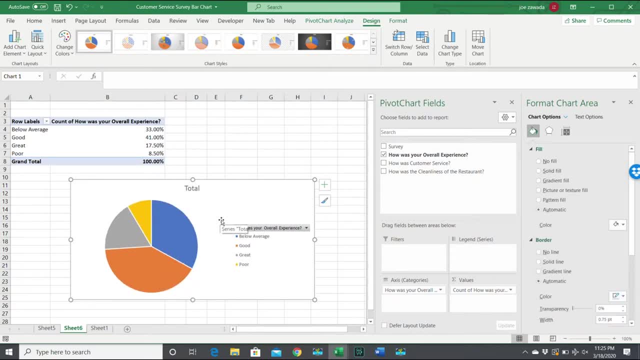 go to hide it here. I'm gonna click on this also and hide that name. and I want to get rid of the legend right here too, because I'm gonna put it right into the actual, into the chart. so I just click down and press delete. so now we got our actual pie chart would click on it. I'm gonna right click and go to add. 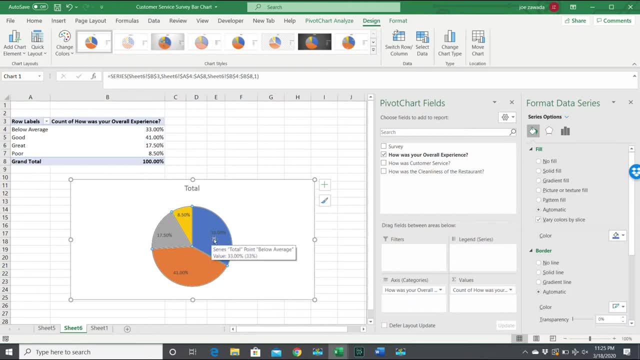 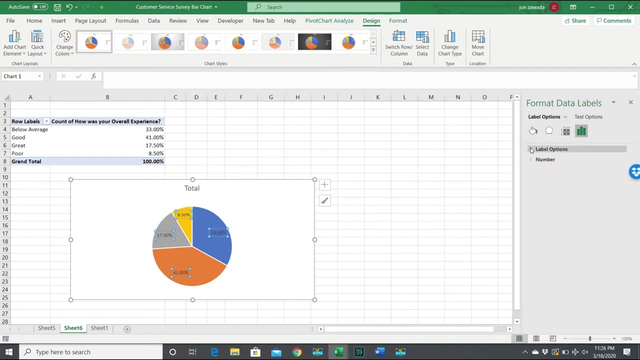 the data labels. so now we have the actual percentages, which is what we want, but let's format the data labels. so we're going over to here and I want to go to this final one for the chart and go to the label options, and we want to put the 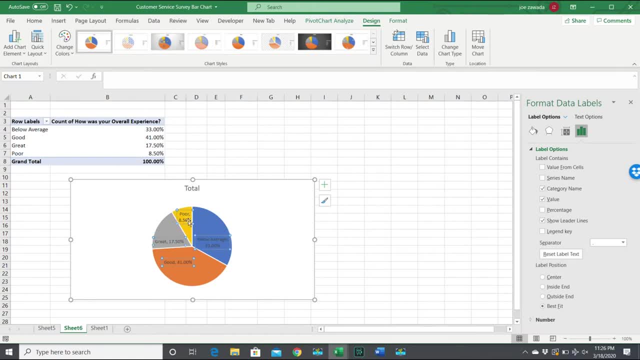 category names also. so then we can kind of see, like, which ones are poor, which ones are great, good, and so on. and I also want to format these a little bit, so I'm just gonna go up to home and make them bold and just make them a slightly bigger. 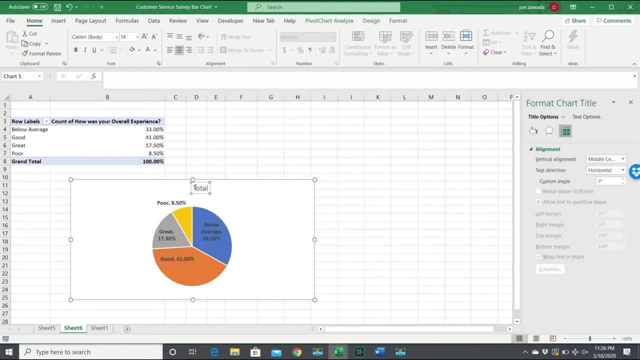 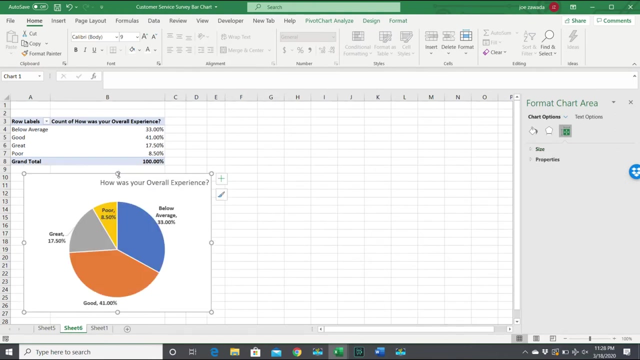 I'm going to change the chart description here and this was: how was your overall experience? so we have the title on here and I'm just gonna okay. so now that we got it a little bit bigger, so make makes it look look a little more clear, and now we can change the type to make it, um, make it look more 3D. so we'll go up to the design. 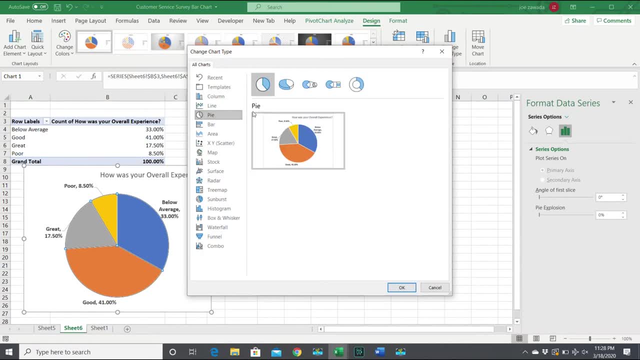 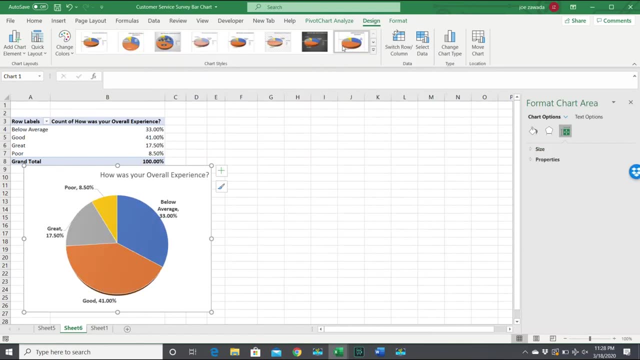 and change chart type and we're going to go to pie chart and let's make it look 3D. so we'll just click the 3D one, click OK and then, once we have it, let's let's look through these ones up here to. 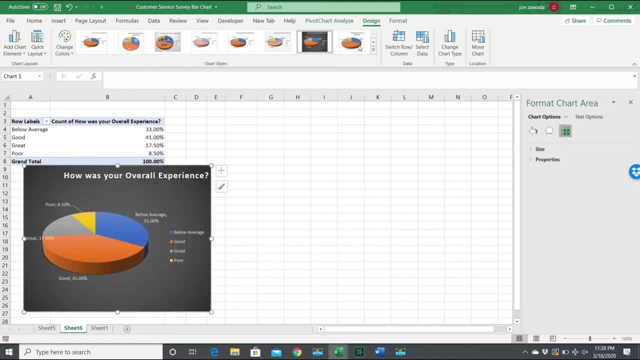 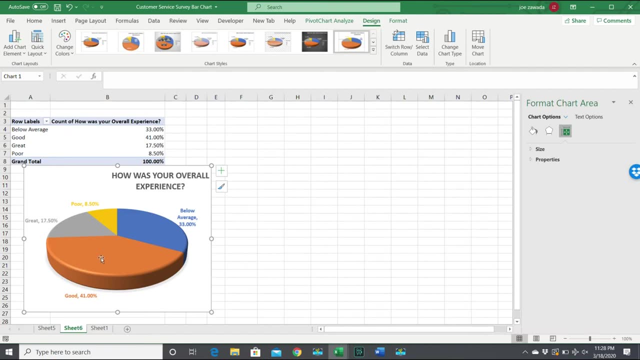 kind of get the one that we want and I kind of like this one. this looks pretty good. it's got your um looks like, looks 3D, almost like a hockey puck. we've got the four different uh titles: good, poor, great and below average. so it's pretty good way to summarize all our data. 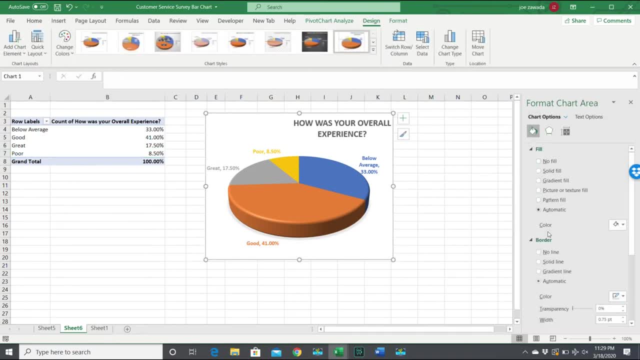 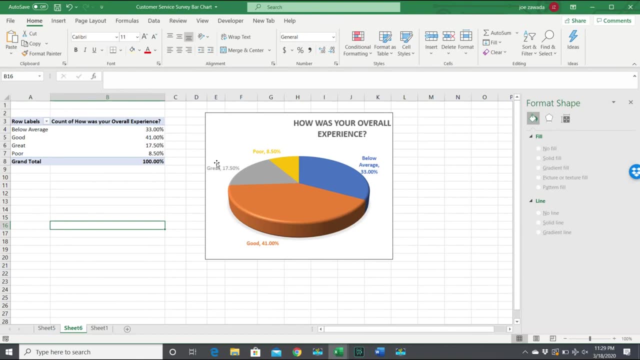 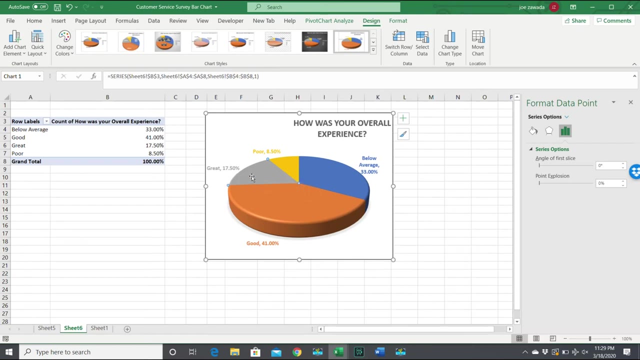 and I think we're pretty good. let me just: I kind of want to format the border, make a stop, put a solid line on the border, and I also want to change the color of this one, because this is the great ones, um, the great reviews, and it's gray. I don't like to cut that. it's gray, so I want to change. 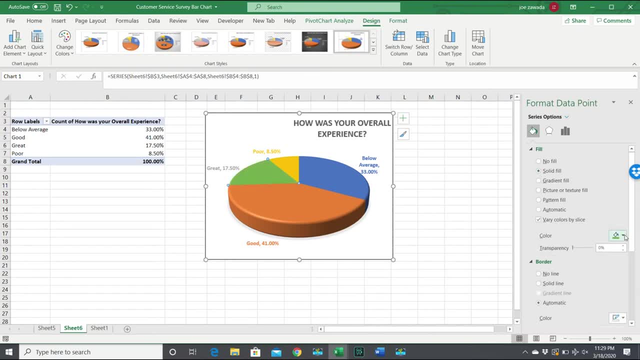 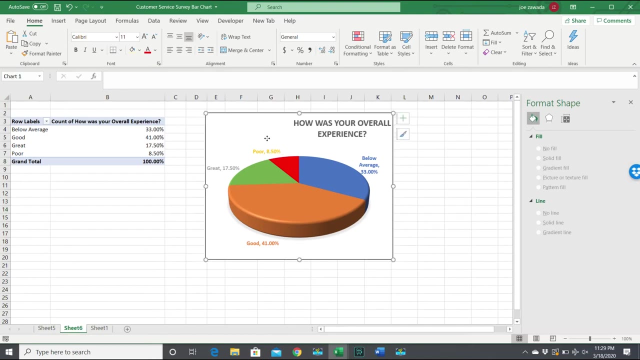 it to a solid fill and green. I actually was going to pick green, so I would like leave it at green and let's change poor to red there. so that's how we can create a chart for it. I'm just copy it, put it right in our data. 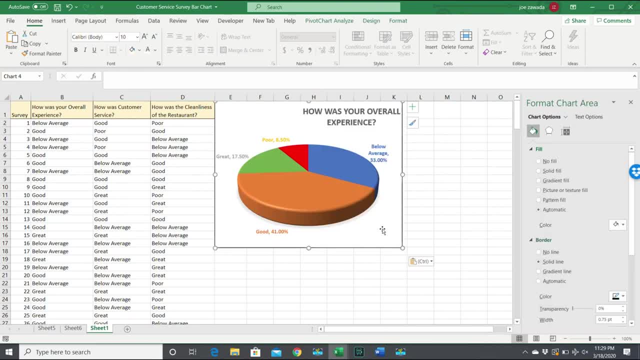 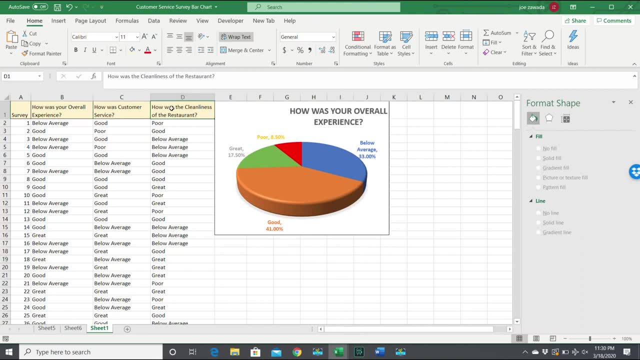 there and we've got our first chart and I'm not going to go through how to how to make the chart for the other ones, because it's the exact same way, but I'll let me just flash fast, fast, fast forward and Show you what the final result is again, and you can just see how you can. 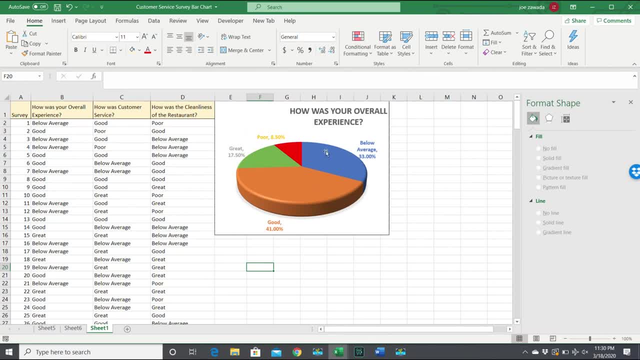 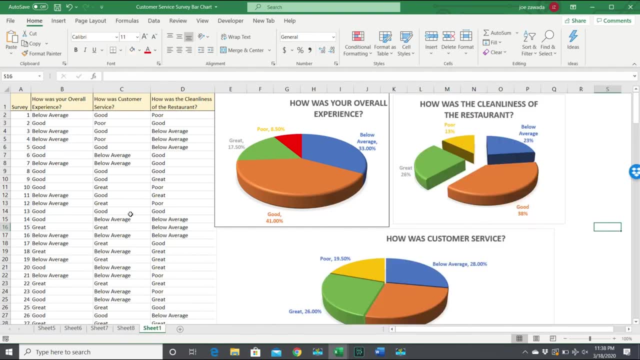 Do a chart like this pretty quickly and get a nice-looking pie chart to show your results of your survey. and here's the final result of the three charts, all set, ready to go and Displaying your information that you want. so Hope this video was helpful and I will see you guys in the next video. 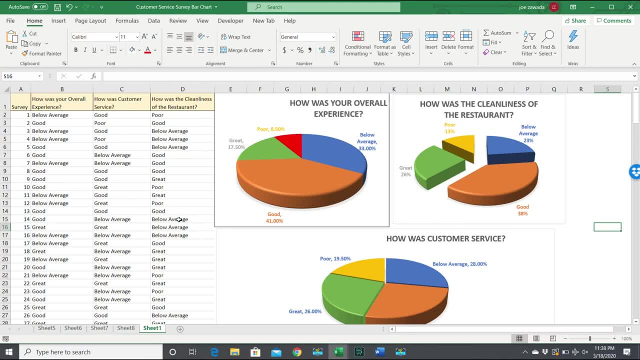 Please click on thumbs up and like the video and subscribe to the channel. Thanks.